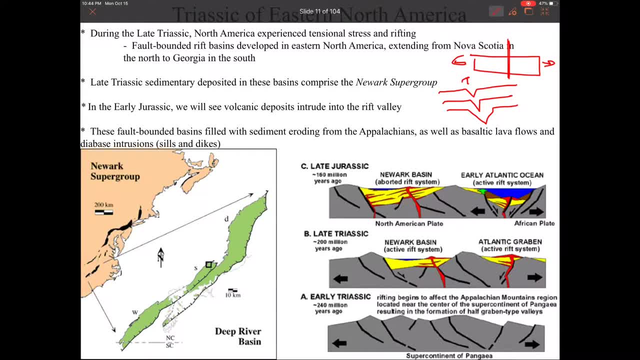 And it starts out in the Triassic, very, not so deep. we get to the Jurassic, we're going to start to see igneous material come into these rift basins. So obviously these rift basins get deep pretty fast. Now what's pretty cool here? so here we are. 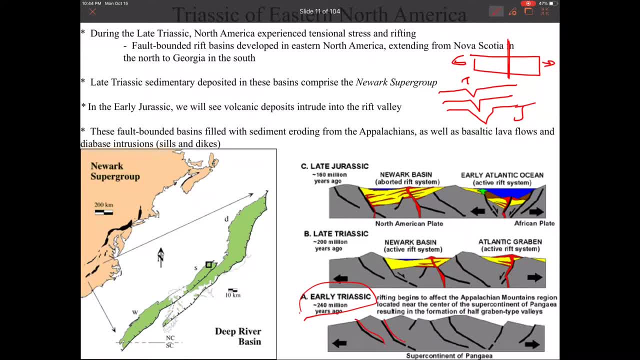 in the early Triassic. you see, we're starting to get these rift, these fault-bound rift basins here and really we have two large basins that are forming. We have the Newark Basin and the Atlantic Basin, which, of course the Atlantic Basin is what eventually opens up right and forms the Atlantic. 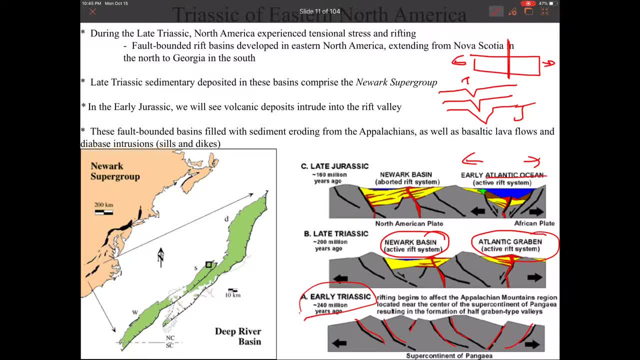 Ocean and the Newark Basin is basically a failed rift. So the rift just kind of stopped. once the Atlantic opened, the pressure was off and that just kept opening. The Newark Basin just kind of stopped so it created this big basin and that's what catches a lot of the eroded material. Remember. 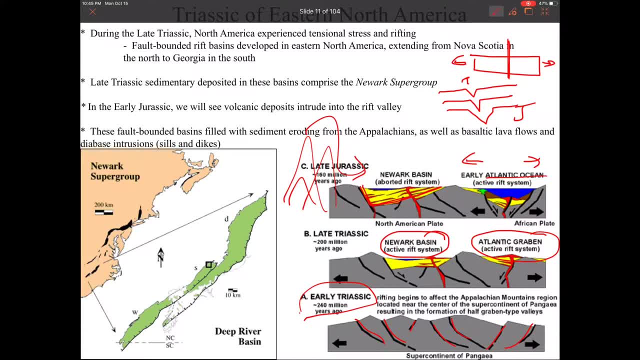 we have mountains over here so that material erodes off and essentially gets deposited in that basin and of course you're going to have lots of water in that basin as well and it makes this rock group we call the Newark Basin, and it's going to be a lot of water in that basin as well and it makes this rock group we call the Newark Basin. 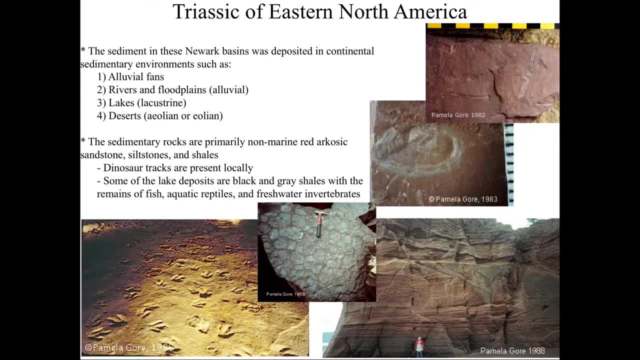 called the Newark Supergroup. So in the Newark Basin we're going to see alluvial fans which, remember, is basically the delta that forms at the base of the mountains right that catches all of that material. We're going to see lots of rivers and floodplains as they flow across that. 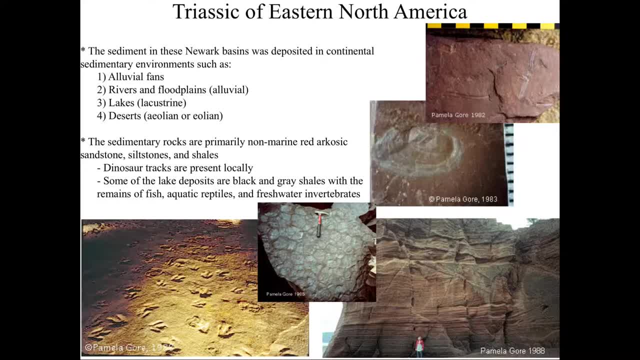 low material or that low part in the basin. We're going to have lots of lakes and lots of deserts as well, which really sets a prime spot here for lots of dinosaur trackways. So as you have lots of river environments, of course dinosaurs are going to go. 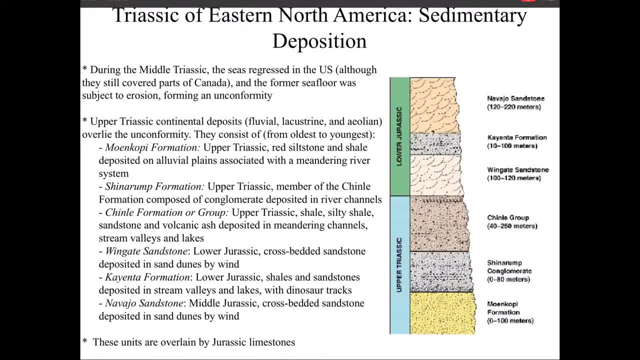 towards the river and we have lots and lots of trackways from this time. But what's really exciting is we have some non-marine deposits that we can find in North America. So these are not ocean-influenced at all. These are all land environments which we haven't seen before. 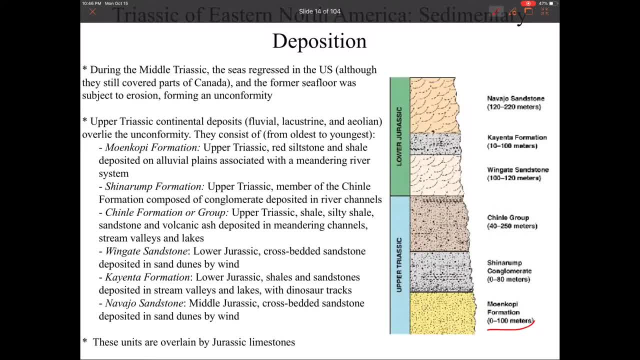 So let's start in the Triassic down here. We'll start with the Menkepi Formation. the Monkepi Formation is basically a river environment where we see silt and shale, this big alluvial plain- okay- and this big river that's just kind of meandering across this large. 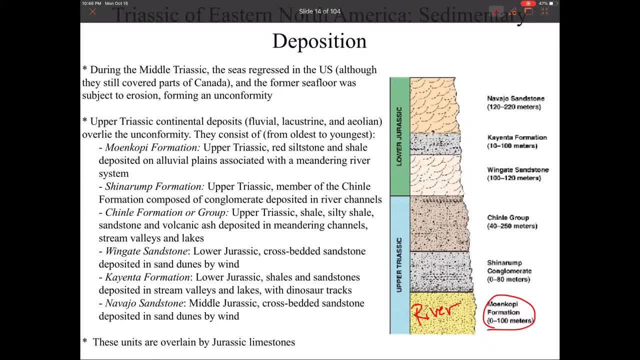 alluvial plain. That's going to be your Menkepi. As we move up in time, we have the Shinarump, which is a conglomerate, so that's a gravel for those of you that haven't taken 101.. So this means that this is. 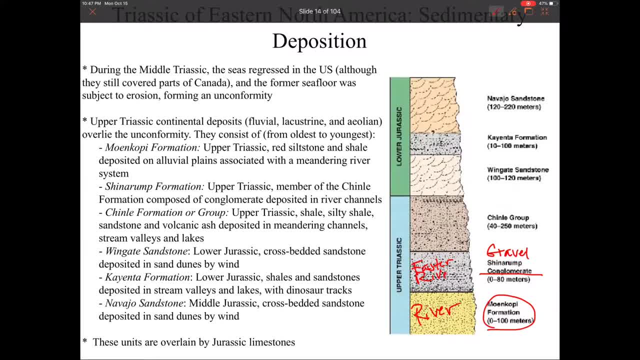 a faster-moving river. Remember, the faster water moves, the bigger grains it can pick up. So as we have a conglomerate there that's telling us that this is a faster river environment, Then we're going to end the Triassic with the Chinle, and the Chinle kind of goes back to what we saw in the Menkepi, where we have this: 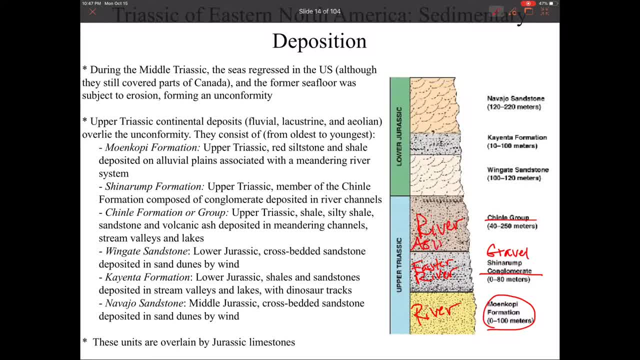 meandering river environment. But this river environment is going to have volcanic ash in it which you can see, that the ash that's going to come in from both the west and the east, as we're going to talk about some of the first orogeny out there, And then, of course, don't. 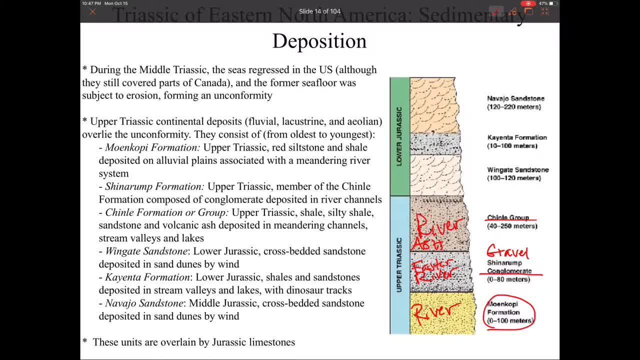 forget. you have the Atlantic Basin opening up as well. Now as we move into the Jurassic, things dry out. We have the Wingate Sandstone, which is just a very large dune environment that's sitting there. Then things get a little bit wetter and we have a stream environment which is the Kayenta Formation, which the 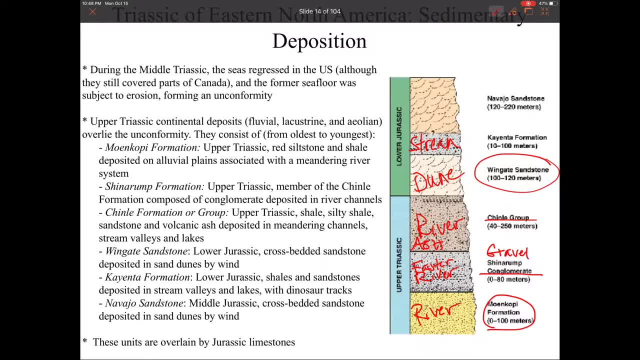 Kayenta has tons of dinosaur truckways all over it, Again showing you this nice fluvial environment, And this is all topped off with the Navajo Sandstone, which are humongous dunes, Basically Saharan-sized dunes. 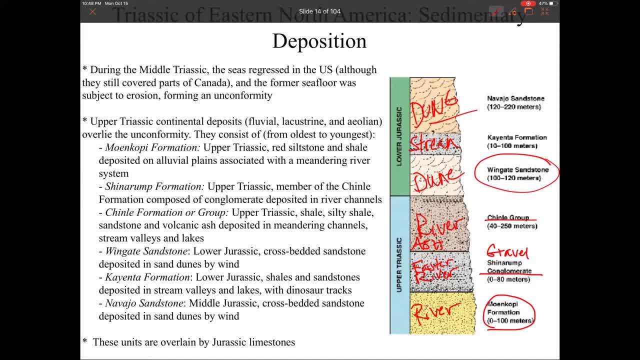 that form at this point. What's actually very impressive is that on top of the Navajo Sandstone we have limestone, Because, remember, limestone is formed in coral reef environments. So this should really impress you with how much and how fast the climate changes. 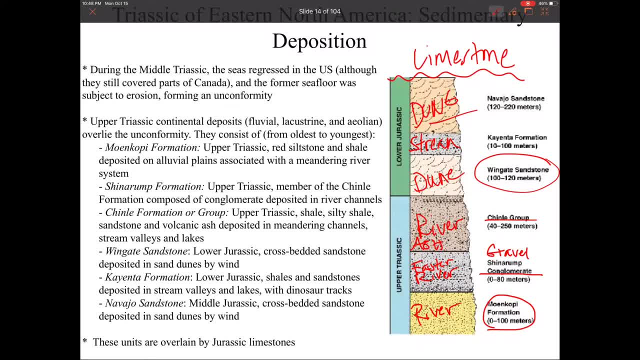 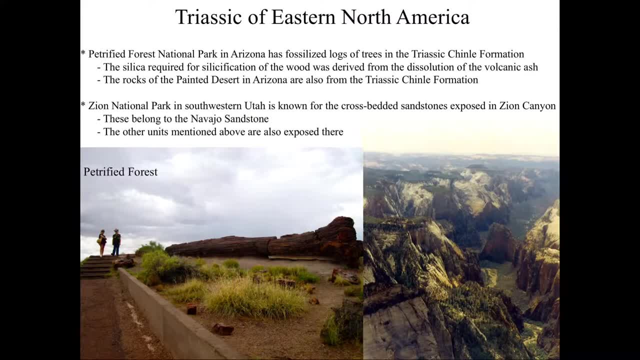 It's really cool to elicit environmental numbers like this. As the's come to shore, we Saharan sized dunes to limestone. That is a huge, huge change. So if we want to see some examples of some of these rocks here, if we want to take a look at the 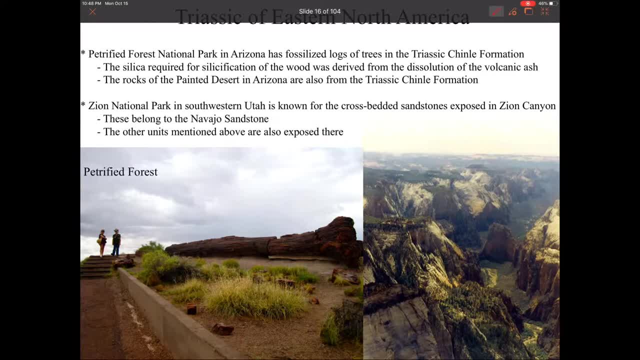 Chinle Formation. we can go to Petrified Forest, which here we have my kid for scale from a very long time ago, But you see we have this really large tree here. So this tree fell into that meandering river and because there was a 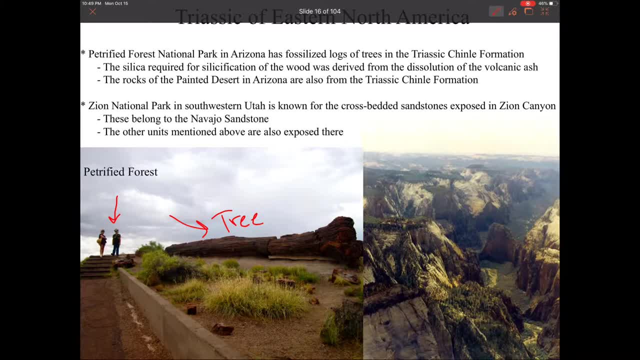 lot of volcanic ash in the water. that volcanic ash had a lot of quartz and as it works its way through the wood, essentially the quartz replaces the organic material in the wood and it slowly turns the wood to stone. right, So producing these petrified trees, right? So basically, they're just, they're there. 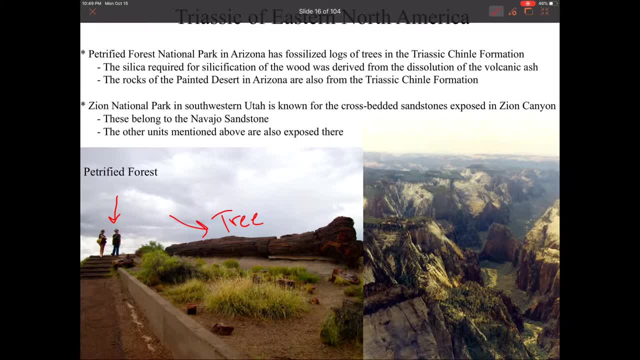 forever. now They've turned to quartz. If you want to see the Navajo Sandstone, you can go to Petrified Forest and you'll see a lot of trees that are growing. You can go to Zion National Park here, which everyone should go to. 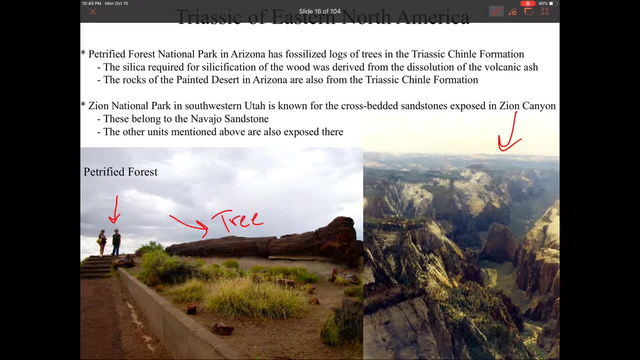 Zion. It's quite incredible. So first to give you a sense of scale, these are large pine trees down here and as you kind of take a look at this, you might notice that there's a basically a lot of triangles. Here you see a triangle with 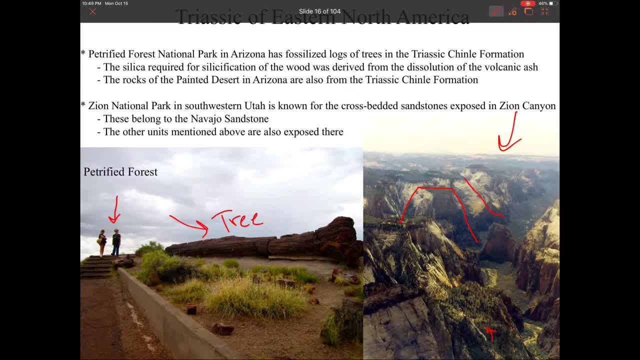 a flat top right Here you see another one, and another one, and another one right. They're all over the place. These are dunes, right? Remember I told you, the Navajo Sandstone? It's basically these large Saharan-sized dunes right that you can see. Oops, sorry. 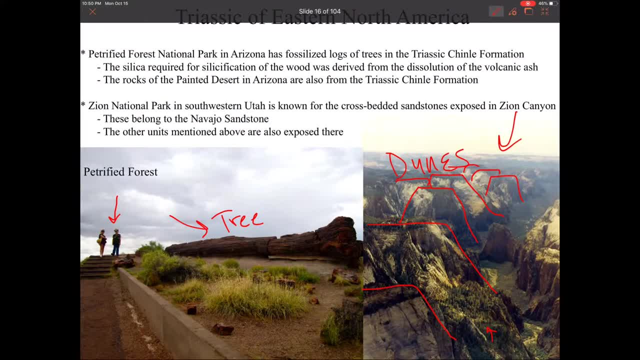 about that: These large Saharan-sized dunes, and they're just full of these huge cross-budded environments. So if you ever get a chance to go to Zion, definitely go, because the sheer size of these dunes is really, really incredible and it kind of gives you. 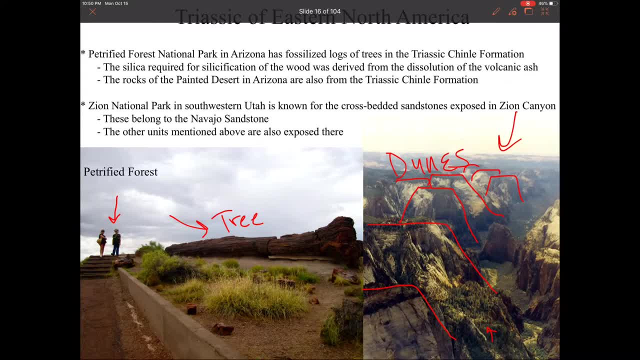 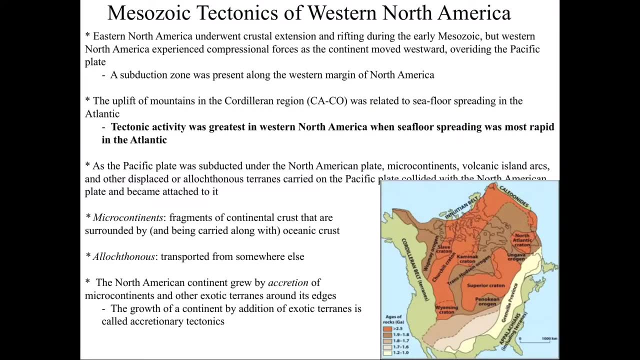 this awesome glimpse of walking back into time and feeling what it would have been like right in the late, during the, you know, Jurassic time period. So what's really important to remember is that plate tectonics ties everything together. So if we remember over here in 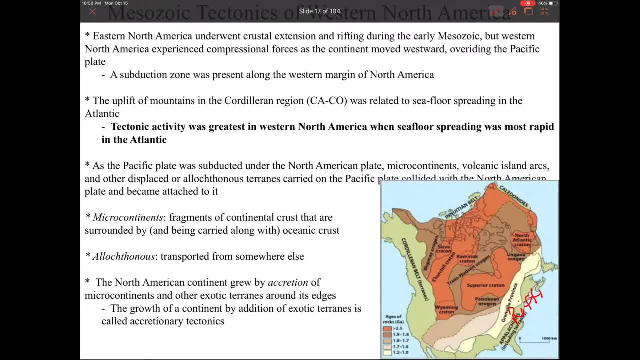 the east. we have rifting going on, So North America's moving this way, Africa's rifting off. okay, So we have divergence. If we're creating new crust in one place, we have to be destroying it somewhere else. We have rifting happening on the east coast and we have subduction happening on the west. 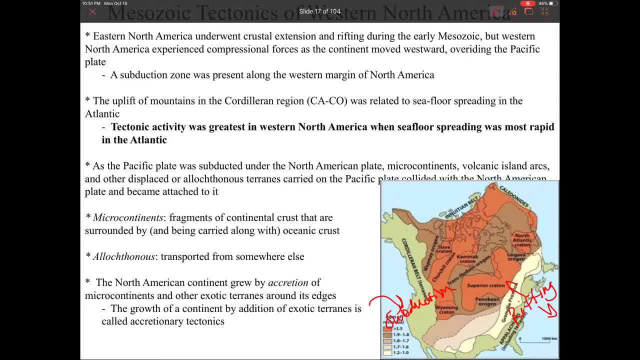 coast okay. So we have to remember that when rifting, when seafloor spreading is happening the fastest in the Atlantic, we're going to see lots of subduction and more tectonic activity in the west. So the faster things spread, the faster things subduct. So it's really 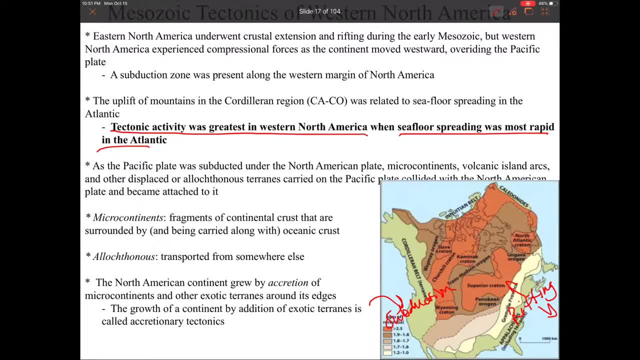 really important to remember that these are tied to each other. So, as this plate is going to subduct – remember we have Pantelassa, which is this huge ocean. Pantelassa is not one big ocean plate, it's made up of multiple ocean. 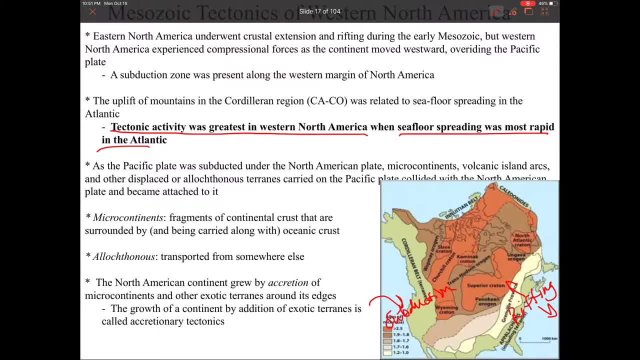 plates, which those ocean plates are colliding with each other and creating large volcanic arcs all over the place. So as these plates subduct underneath North America, it's going to bring in lots of island arcs, microcontinents, these things we call aloxanous terrains, which are our pieces of crest that have been 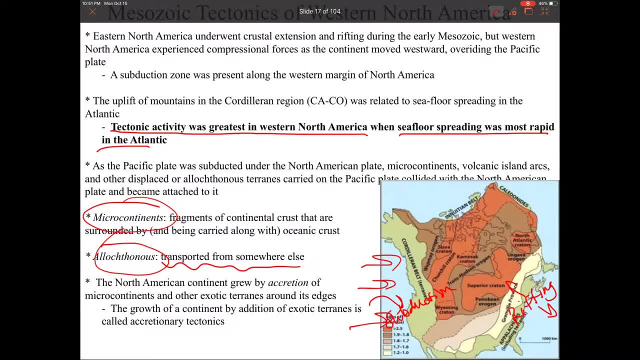 it's ported from a far away and they're going to come in and they're going to collide with the western part of North America And this is really what's going to generate the Cordillera, everything going from the western part of California all the way into the Rocky Mountains in Denver. 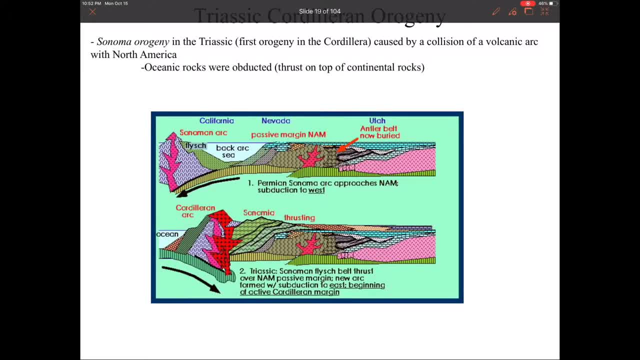 So we see our first orogeny of the Mesozoic occur. So remember, the ablations are done, forming. at this point They're not going to form anymore, They're only actually going to erode. So if we look at the Cordillera, we've actually already seen our first orogeny. Remember that occurred. 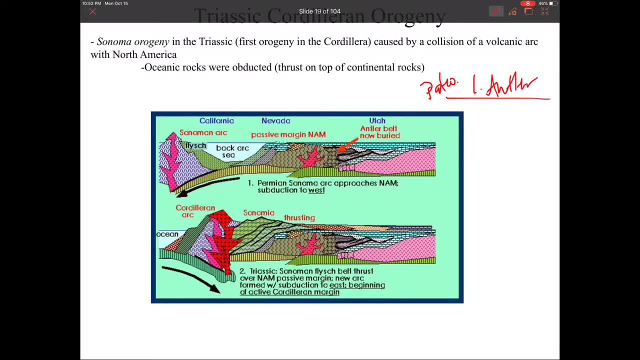 in the Paleozoic That was the antler, And in the Mesozoic we're going to see four more orogenies occur. So this next one is the Sonoma And the Sonoma orogeny. remember we have these large. 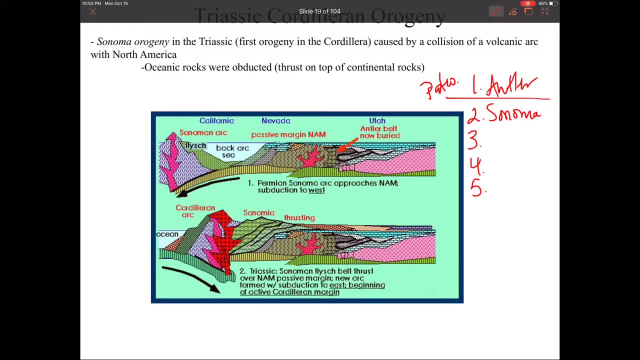 island arcs that are out there. I know this picture is a cross-section so it just looks like one volcano, But remember it's a whole line of volcanoes right that are approaching the western edge of North America. So as this line of volcanoes comes in and collides, 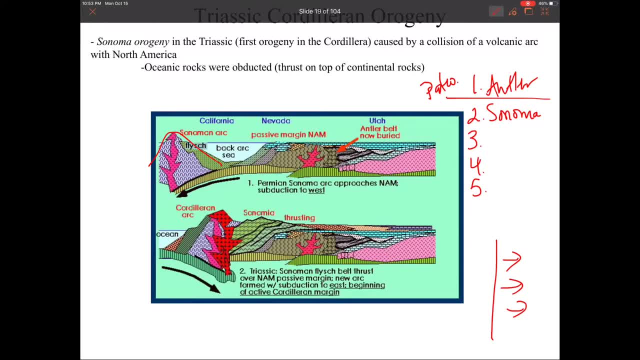 it collides in with such force. this should really impress you that the seafloor that was sitting here in between North America and the island arc, instead of getting subducted, it gets crunched and tossed up onto the continent. We call that abduction, So you can actually see the ophelite.